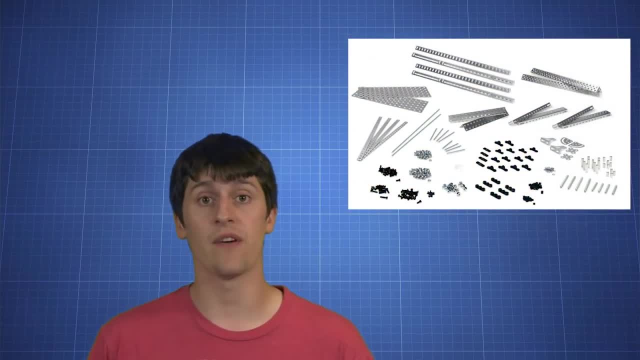 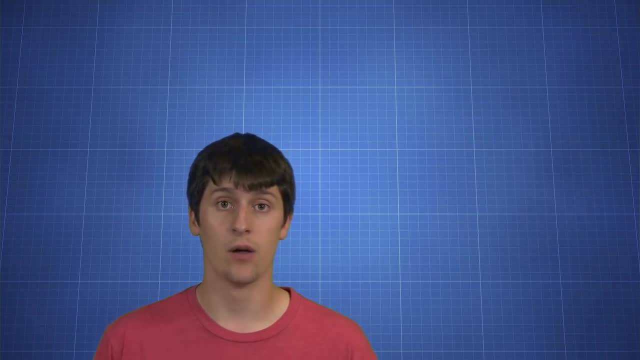 Structural parts are what hold your machine together or that provide support to particular parts. There are quite a few structural items, so we're not going to go through all of them right now. We're just going to touch on the most important parts. The four main types of structural parts are: L channel. 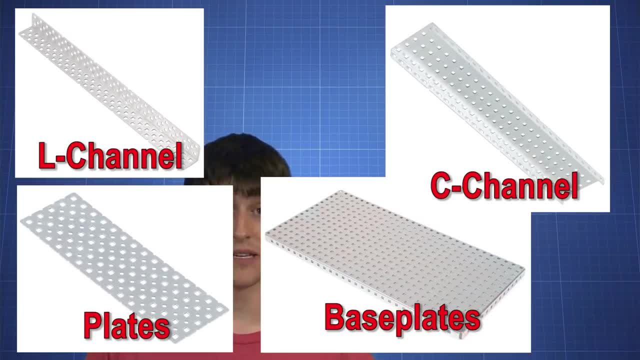 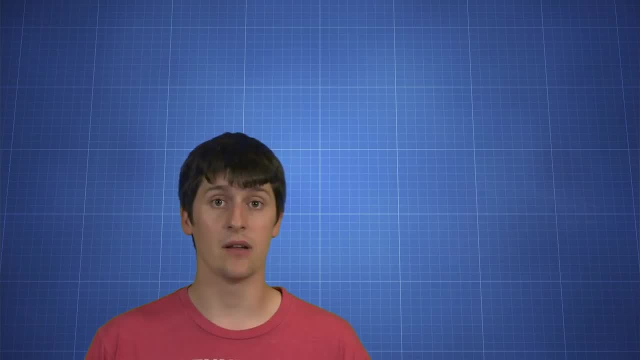 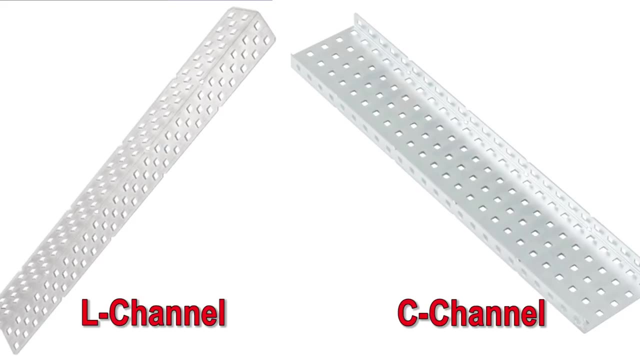 C channel plates and base plates. Many people get basic structural parts confused in VEX kits, so let's talk about channel pieces. C channel pieces and L channel pieces are often confused. If you look at the bracket along the edge you'll see whether it's a C bracket or an L bracket. It's pretty straightforward. 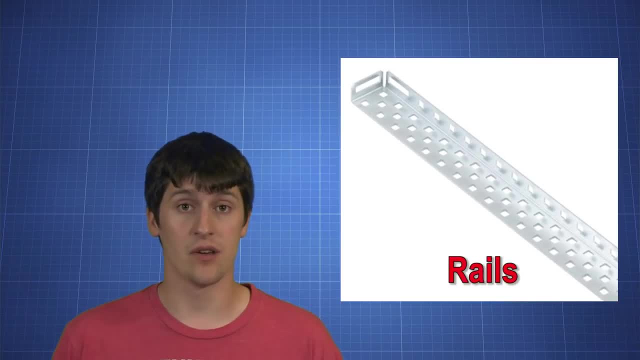 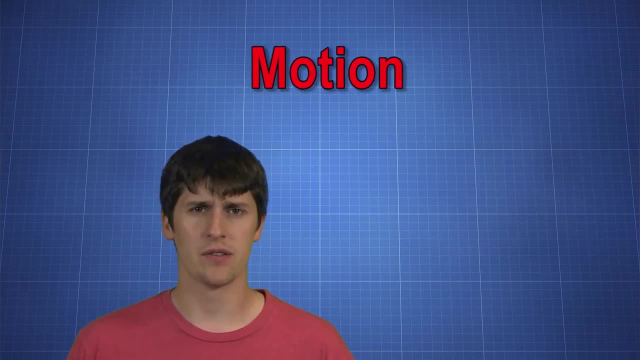 There are some L brackets that have ends on them- flat ends- so that you can attach them to things Those are called rails. Let's move on to motion parts. Motors and servos are little box things that you can attach to your machine. They can be used. 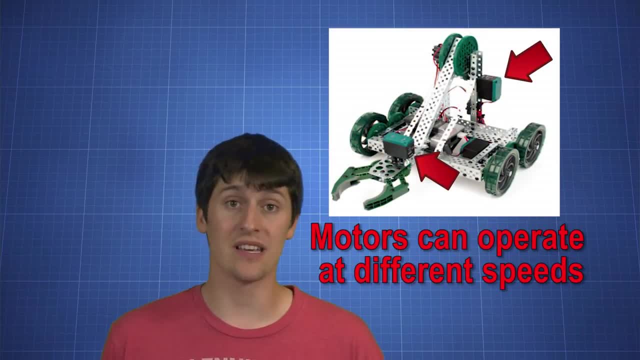 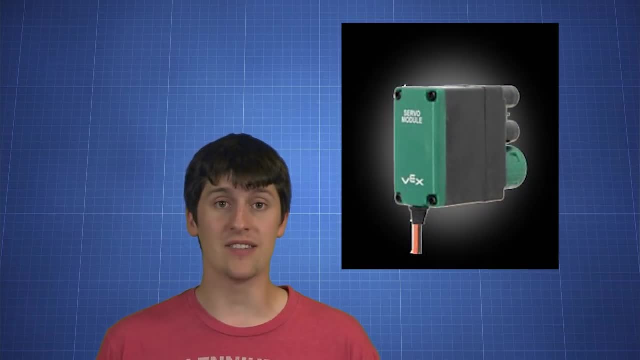 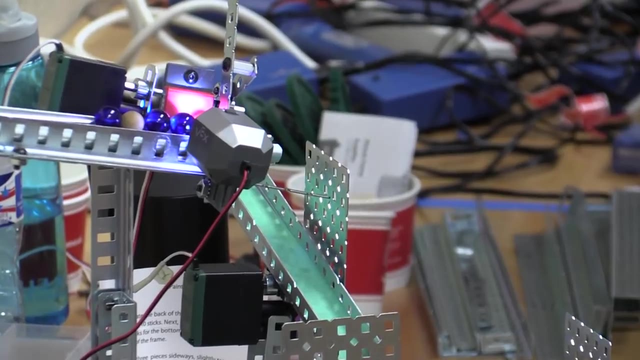 to help your device move or to spin a gear or a sprocket. Servos are a little different than motors. They are smaller and instead of having a changing speed motor, might servos actually snap to angles? They can be used to adjust the 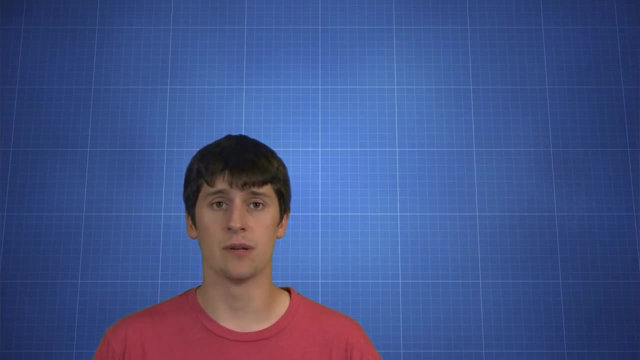 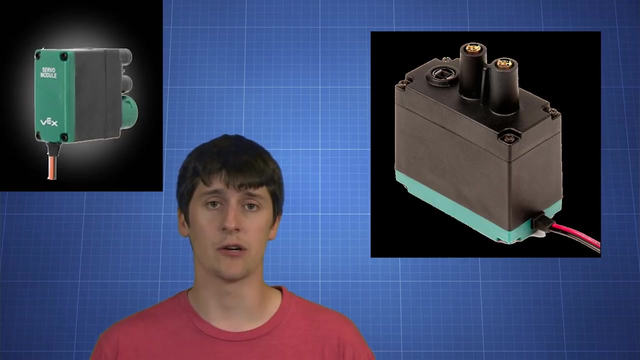 angle that something is at. They're really good for precision instruments. To tell a motor from a servo, you just need to look at the size of the box. Servos are a lot smaller. They also say servo on them. Gears or sprockets can be used to. 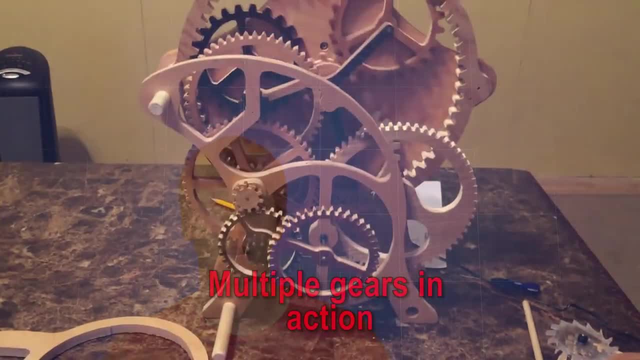 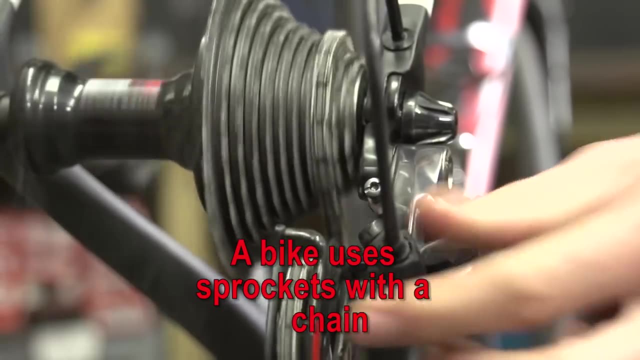 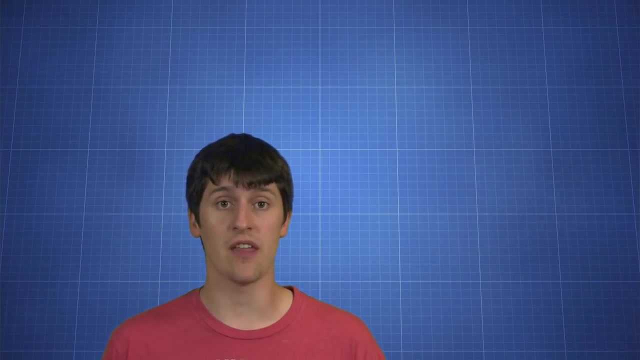 rotate things. You've probably seen a gear before in a watch or maybe a clock tower, but you may not have heard of a sprocket. You can see a sprocket if you look at a bicycle chain. There are multiple sprockets that are being used on a bike. If you put multiple gears together, you 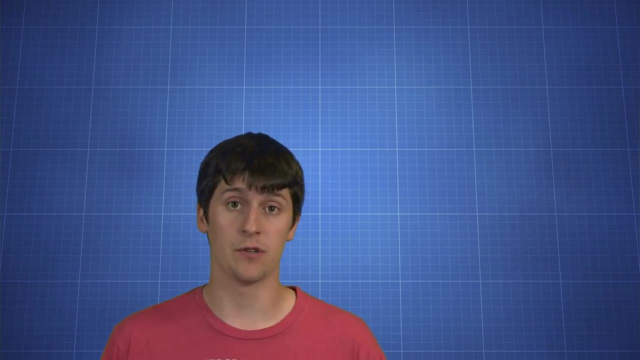 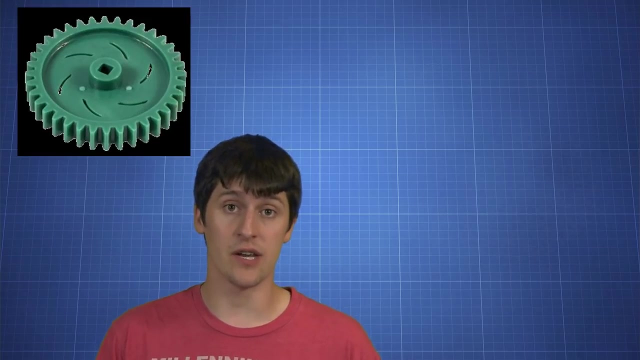 get what's called a gear train. Multiple gears and multiple sprockets are a little complicated so we're not going to talk about those right now, but we will come back to those later. A lot of people confuse gears and sprockets. The 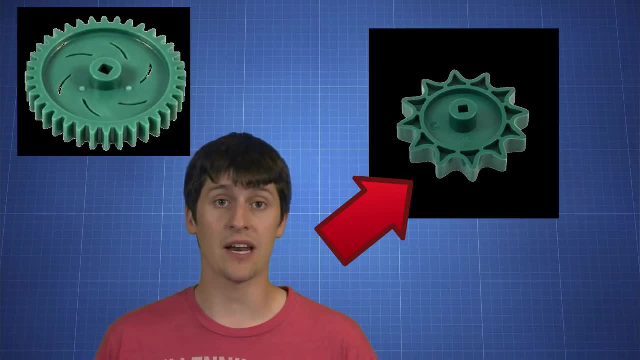 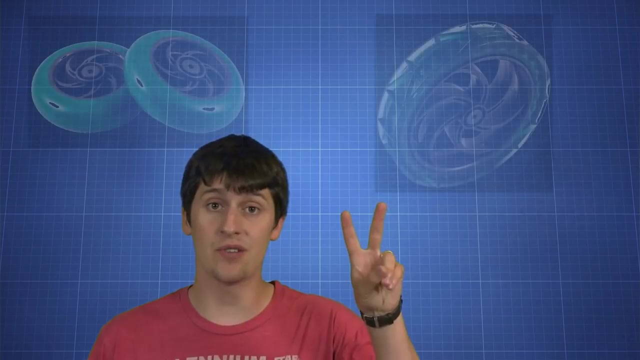 difference is pretty simple. Let's look at a sprocket. A sprocket has much taller teeth and the teeth are a little bit farther apart. Teeth also tend to look a little swooped or they have a dip between the teeth. Moving on, Our Vex kits come with wheels. There are two types of wheels in the Vex. 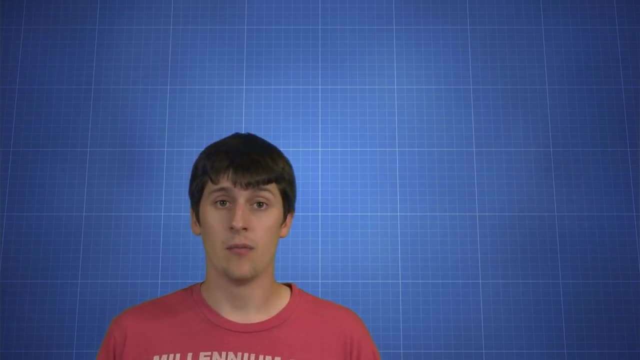 kits. Not really going to talk about wheels a whole lot, but picking a type of wheel just depends on what you want your device to do. Gears or sprockets can be used with chains or treads. You've probably seen treads before on a tank. 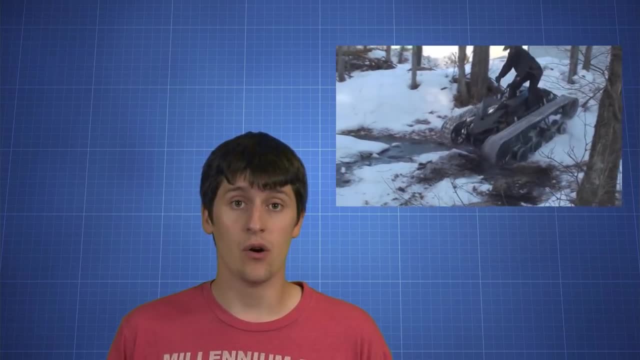 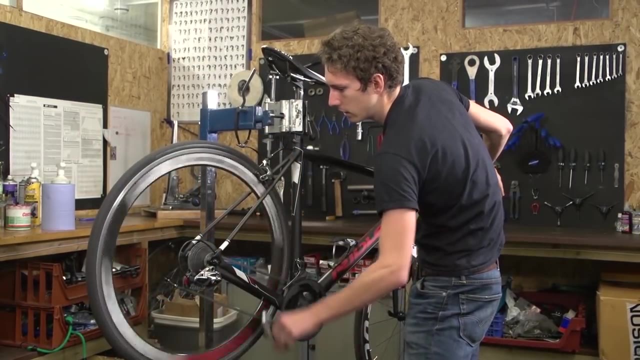 They can be used to move your object- that's true- or they can be used like a conveyor belt. Chains tend to be used to move your object. Move energy from one place to another, like your bike does. Your bike translates the energy from your feet to the back wheel using a chain. Whichever motion. 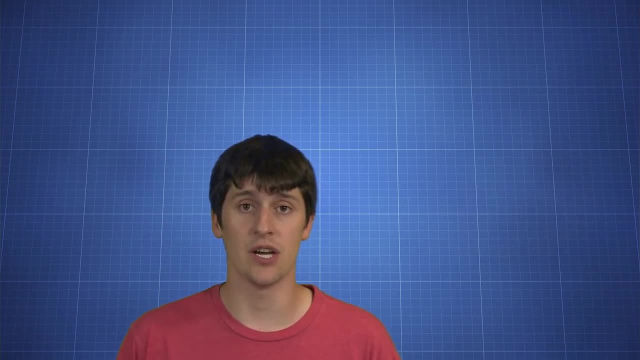 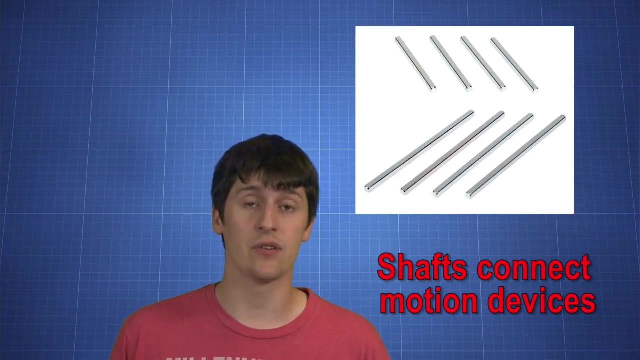 device you're using, you're going to need to attach it to your machine. To attach a motor, a servo, a gear or a sprocket to your machine, you use what's called a shaft or a drive shaft. Just like motion, the electronics category makes up a. 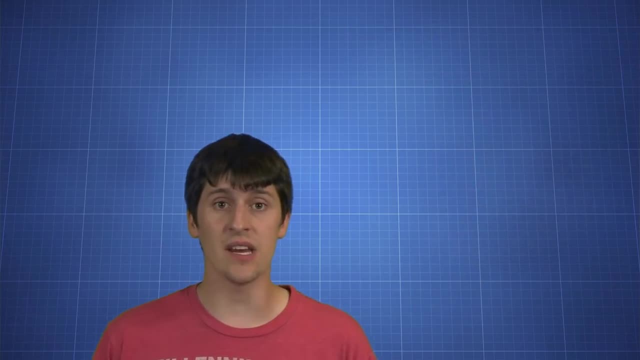 bunch of the parts that are in our Vex kits. The single most important part in the Vex kits is called the cortex. Think of the cortex as the brain of your machine. You will use your cortex to connect your motors, your sensors and 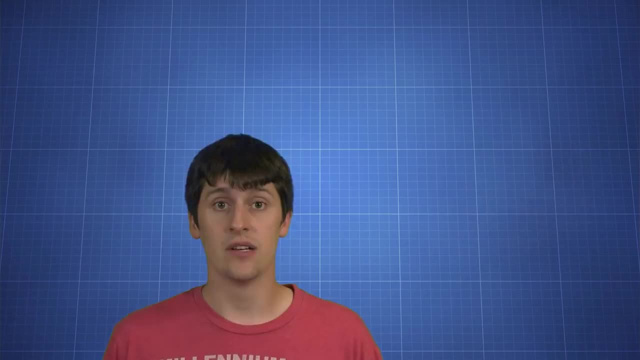 your servos or anything that uses electricity, to the rest of your machine. It's going to provide power to those things and it's going to tell them what to do, based on a program that you write and send to that cortex. Now, since the cortex is using electricity, it needs a power source. All of our cortex have a. 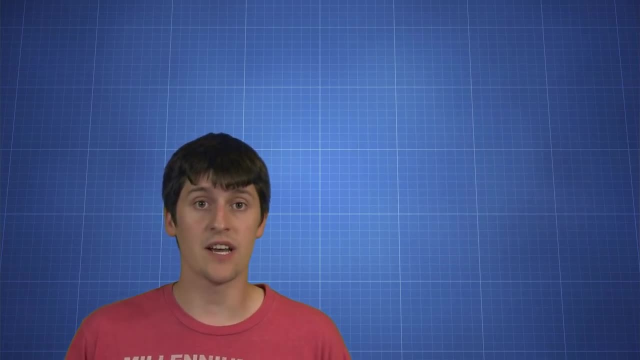 special battery that we use to attach to them. Cortex's can also be used with a controller, a special controller that is provided by Vex. If you want to use the controller, you need to use a wireless USB adapter. Of course, that means that you'll need to program your controller. 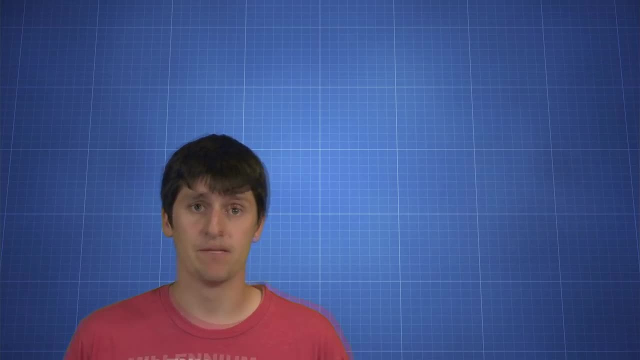 and well, that's not exactly as easy as it sounds. Sensors are a really important part of our project. Oftentimes you'll find that you need to measure values in order to make your machine work correctly. There are two types of sensors that we use in Vex: Analog and digital. 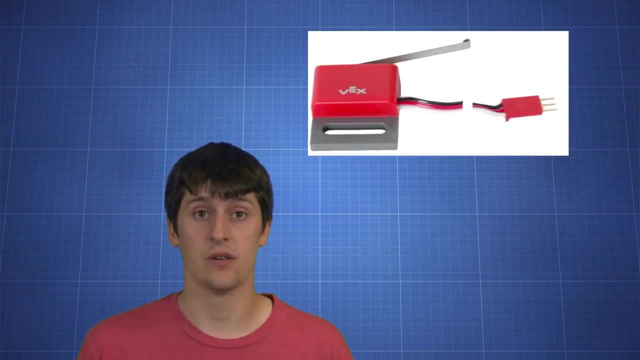 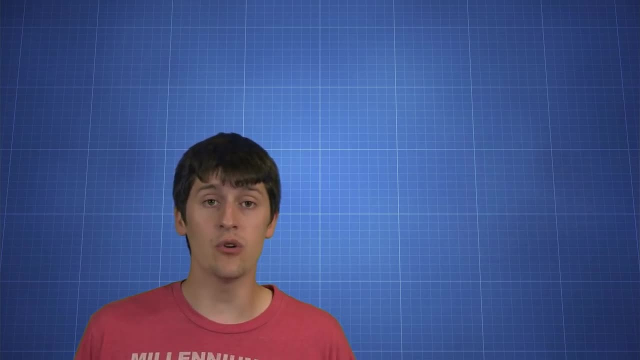 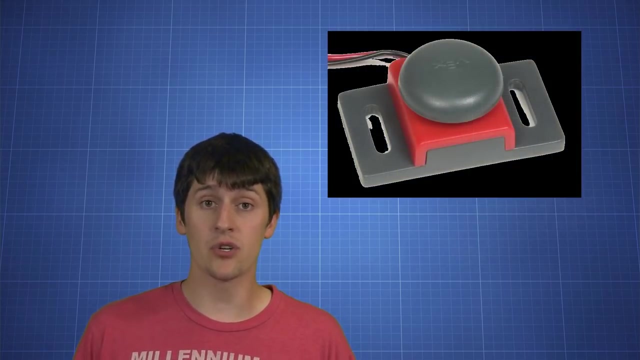 Digital sensors read one of two values. They'll either read a 1 or a 0. It's either on or off. Computers only understand a 0 or a 1.. So if you use something like, say, a bump switch, if you push the button the computer reads a. 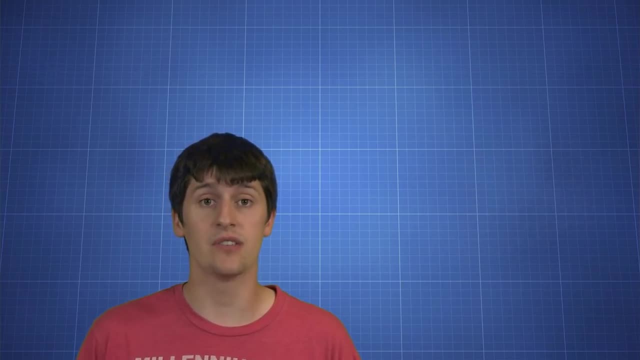 value of 1.. If it's not pushed, it reads a value of 0.. Analog sensors can read a range of numbers. So an analog sensor could have a value of 20 that it reading, or it could have a value of 600.. The last type of Vex equipment that we 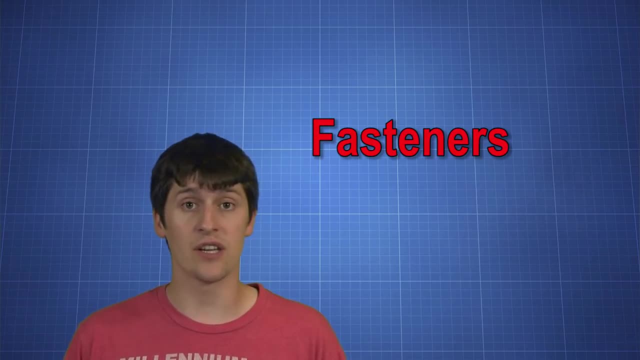 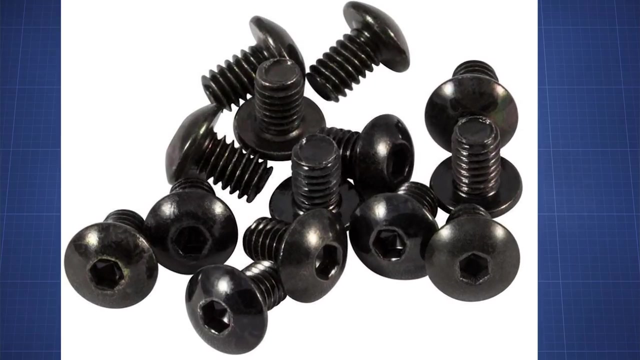 need to talk about is fasteners. Fasteners are often overlooked, and they're really important. They are what hold your device together. Vex uses what's called a hex head for their screws, which means that a standard Phillips or a flathead screwdriver doesn't work for them, So we have special 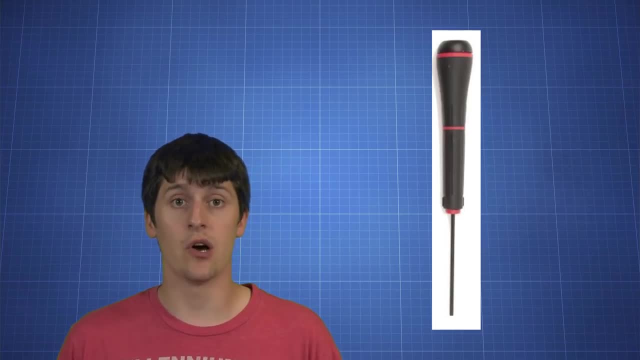 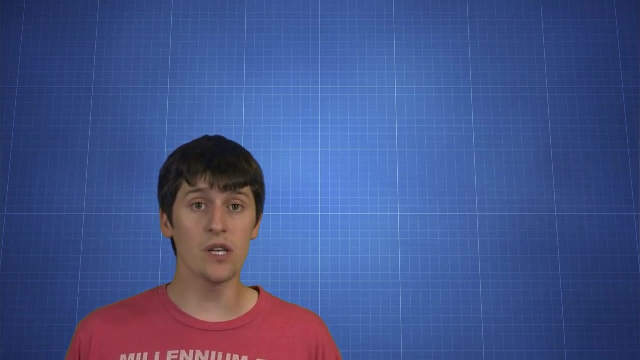 screwdrivers that we use to install screws on our machines. Screws probably aren't new to you, but we do have a lot of different sizes of screws, so it's really important to keep our screw kits organized. Most of our screws work on almost every piece of equipment, but 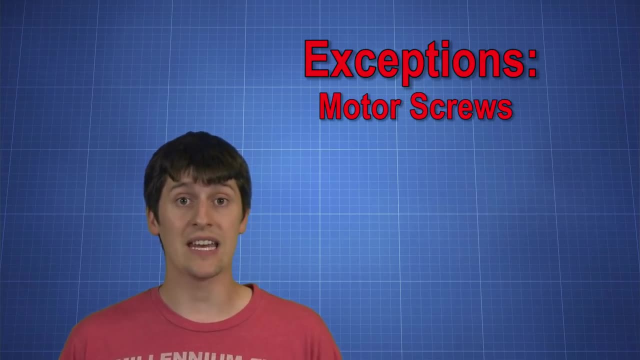 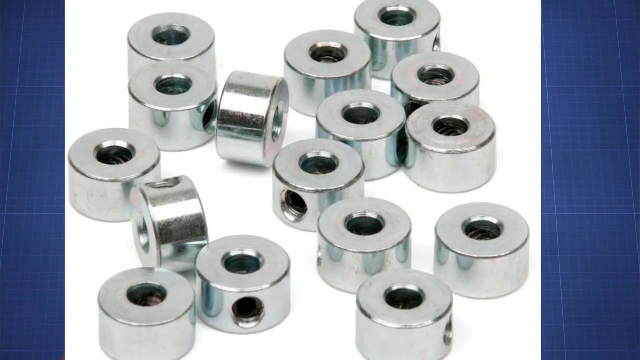 there are a couple of exceptions: Motor screws and collars. Collars are not screws. Collars attach to driveshafts to hold things in place. For instance, if I'm attaching a motor to a wheel, I'm going to use multiple collars to keep. 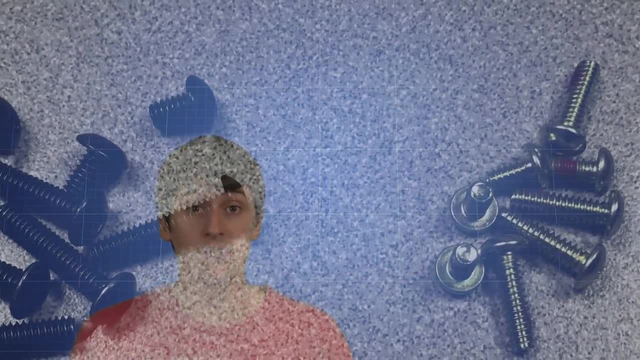 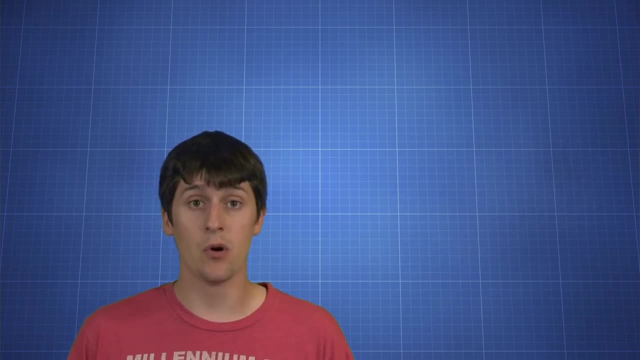 everything steady on that driveshaft. Motor screws are special screws that we use specifically for fastening a motor to a wheel. Motor screws are mostly gold. Your kit might have some black motor screws in it, so if you're trying to install a screw on something and the screwdriver isn't 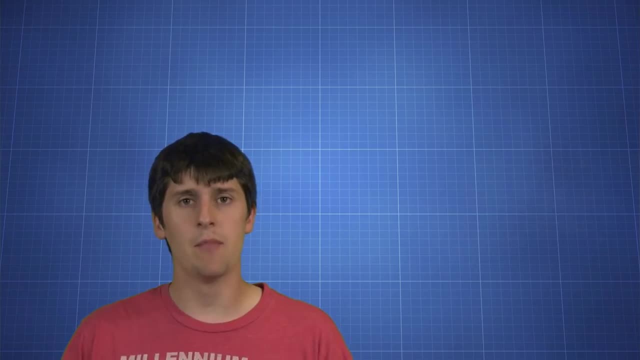 working. you're probably using the wrong kind of screw. Collars and motor screws both use the smaller head of hex, so it's really important that, if you're installing a machine, that you have two types of screwdrivers available so that you can switch in between. It's really, really important that your group takes 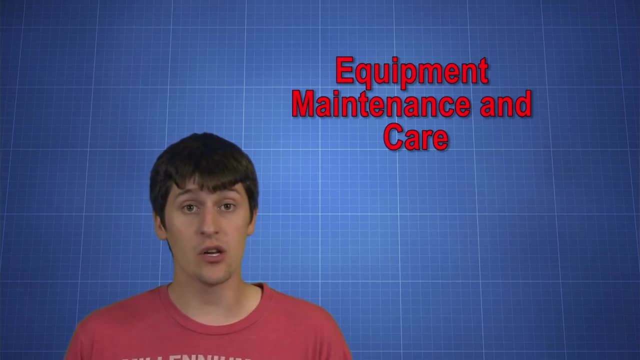 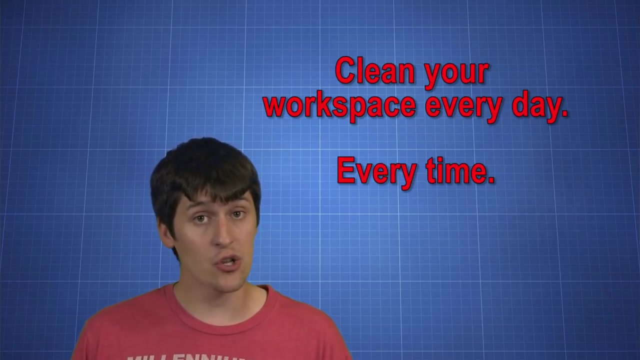 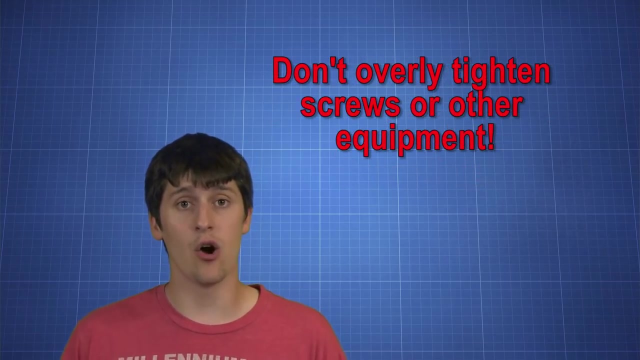 good care of the equipment that you're using. This includes proper storage, putting things in the appropriate place, cleaning up your area, making sure that you haven't dropped anything on the floor. you shouldn't bend any parts without permission, and it's really important that you not over tighten. 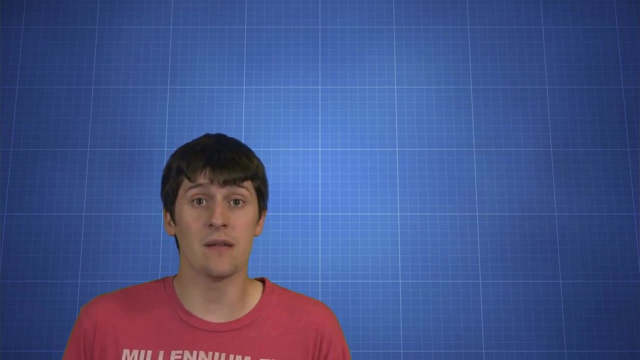 screws on equipment Over tightening parts can make them seize up and make multiple parts unusable permanently. When you handle motors or sensors, you need to take caution with the power of the motor. If you're using a motor that's not connected to the motor, you're probably using the pins that attach to the cortex.